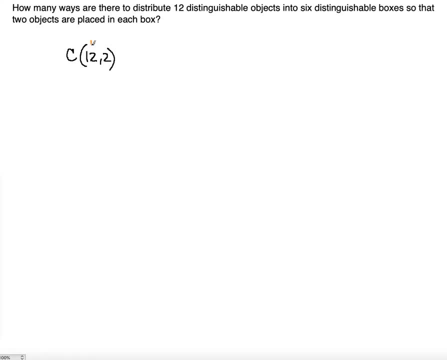 NCR, in which N is equal to 12 and R is equal to 2, right? So NCR is going to be 12. choose 2, 12, combination 2.. So now the product rule states that we will multiply the next combination, right. 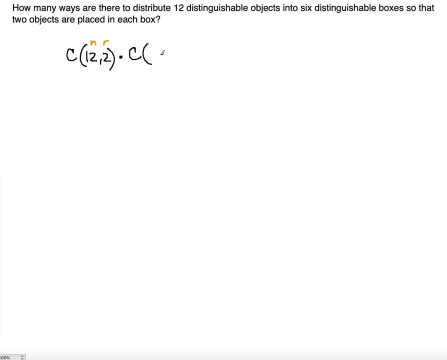 for the second box. In the second box we have 12 left right, Because we already chose 2 for the first box. The second box will have two guys chosen, two objects chosen from 10, right, So it's going to be 10. choose 2 and then the third one will be the combination. 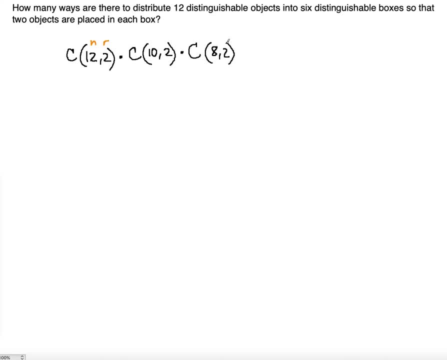 from the eight, choose 2, right, Because there will be 8. and from the fourth box- there will be 6- choose 2. and finally, from the last box, for the last box, it's going to be well, actually, it's going to be 6.. 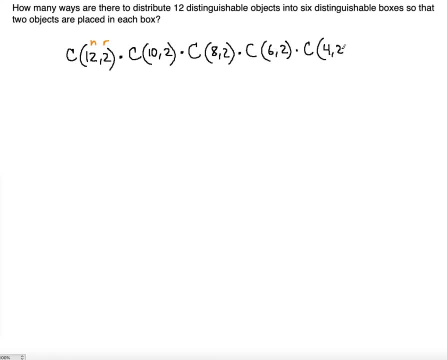 that's not the last one, this one before last, so it's gonna be 4 choose 2 and then finally 2 choose 2. okay, so the product rule makes sense, because when you're talking about permutations, I know this is a combination, but combination comes from the permutation and the permutation is the ordering of selected. 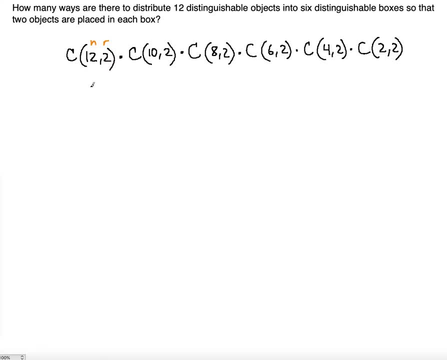 objects. but in this case the combination makes sure there's no ordering, that there's simply a combination, let's say two distinguishable objects. once they're chosen, you're not gonna order them within the same box, right? so that's what the combination takes care of. so what this? 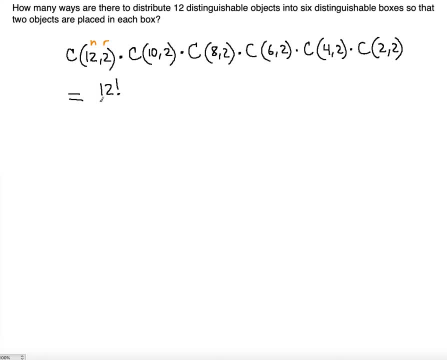 means is that we're gonna have 12 factorial divided by the 2 factorial and then also, so the 2 factorial is accounted for by this 2 that you see here, the r-value, but also it has to be n minus R, remember n minus R factorial is going to be 12 minus 2 factorial 12. 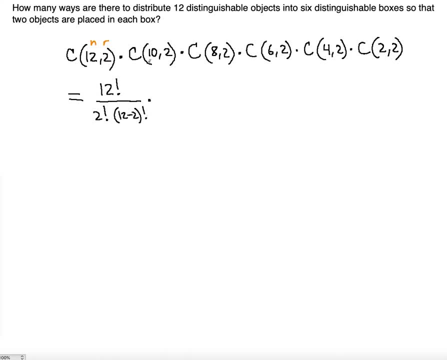 minus 2 factorial multiplied by 10 factorial, that this number divided by the 2 factorial, and then the difference between 10 and 2 factorial, which is 8 factorial right, and then 8 factorial for the third box, divided by the 2 factorial, and the difference between 8 and 2, which is 6 factorial times 6 factorial divided. 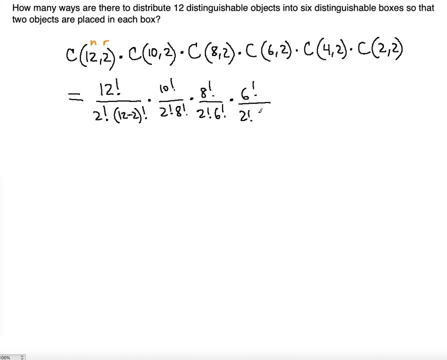 by- sorry- 2 factorial and then 6 minus 2, that's 4 factorial multiplied by 4 factorial divided by 2 factorial and the difference, which is 2, between 2 and 4 factorial times the last factorial, 2 factorial divided by the 2 factorial, the 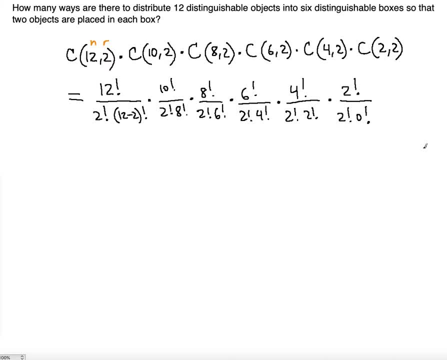 right number divided by the difference, which is 0 factorial, and, as you know, the 0 factorial is equal to 1. okay, so so, as you can see, look what have, look what's going on here- we can actually cancel out the 10 factorial, the 8 factorial, the 6. 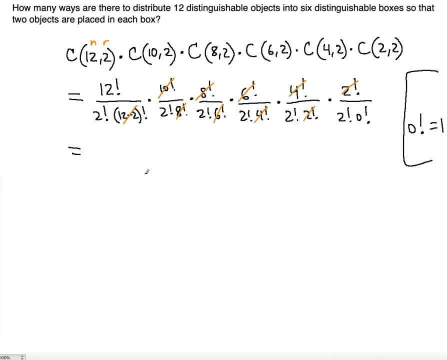 factorials, the 4 factorials, the 2 factorials. so in the end, all we have left is 12 factorial divided by the 2 factorial, 2 factorial. how many twos are there? factorials 1, 2, 3, 4, 5, 6. 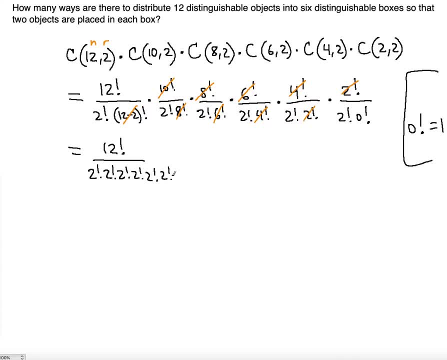 1, 2, 3, 4, 5, 6 right and the 0 factorial is equals to 0. so what does that mean? it means that essentially, for each distinguishable object we'll take one spot right in any box that you choose. so that means that you essentially can: 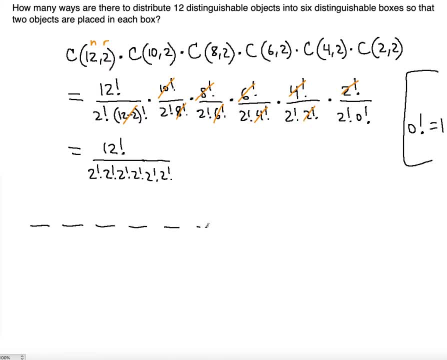 choose 12 spaces: 5, 6, 7, 8, 9, 10, 11, 12. right 12 can go for the first one, then 11, then 10,, then 9,, then 8,, then 7,, 6,, 5,, 4,, 3,, 2, 1.. 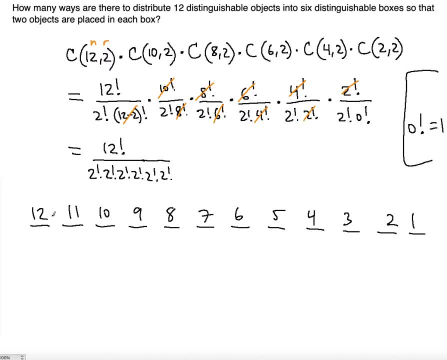 But this would be permutation right. This, when multiplied, would allow you to order these right. Ordering in each box will take place, but the bottom that you see here makes everything turn out to be a combination rather than a permutation, because you're also dividing for each box. 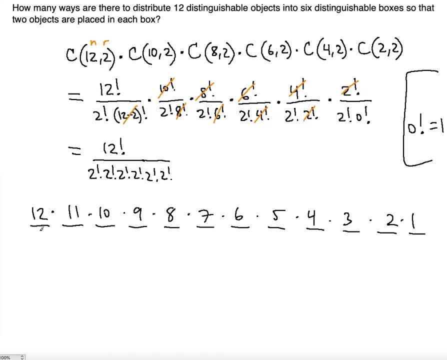 You're having the division by 2 factorial. because you're not going to order the first 2 in the first box, You're not going to order the second 2.. You're not going to order the third 2.. You're not going to order the fourth 2 in the fourth box. 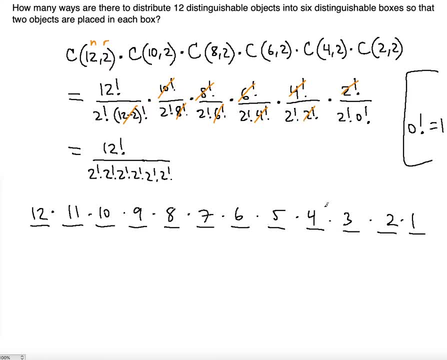 You're not going to order the fifth box 2 that you choose, right, You're not going to count distributing, let's say, the first object in the first box and then the second object, and then saying, but wait, there's another way. 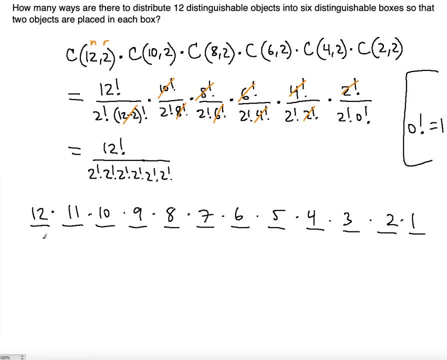 We can take the second object first and then place the first object. No, that's still one way, right? That's why these 2 factorials take care of that right. It's not a permutation, This is a combination, right. 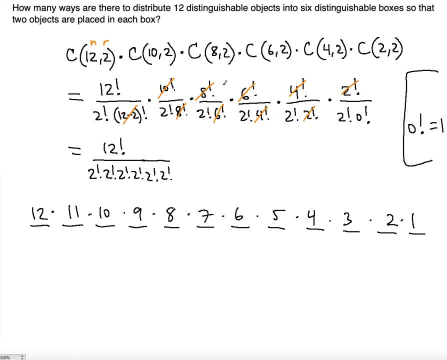 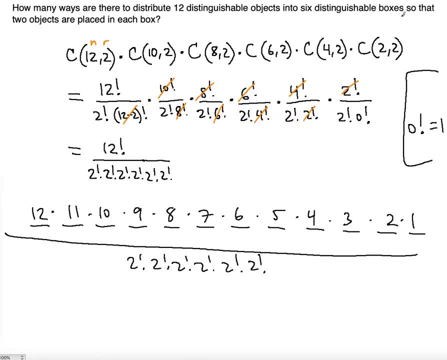 They just make sure that in each box, in each of the 6 distinguishable boxes, you don't have ordering of the 2 distinguishable objects in them, right? So this equals 12 factorial. Let's see what that is on the calculator. 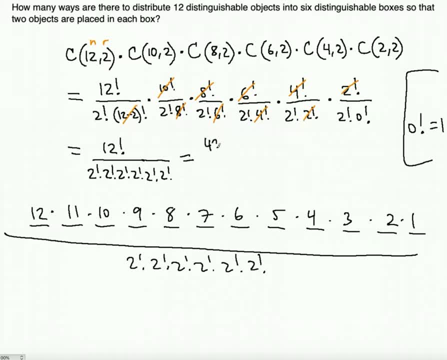 That's going to be 479 million, That's going to be 1,600 divided by 2 factorial raised to the sixth power, And 2 factorial is simply 2 times 1, which is equal to 2.. So 2, and there are how many 2's? 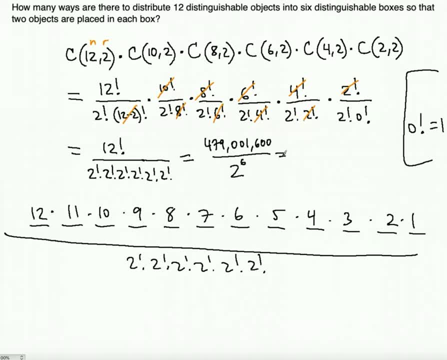 Six of them, right. So it's raised to the sixth power. So if you do that and you divide it by the 2 to the sixth power, you will get 7.. 4, 8, 4, 4, 0, 0, right. 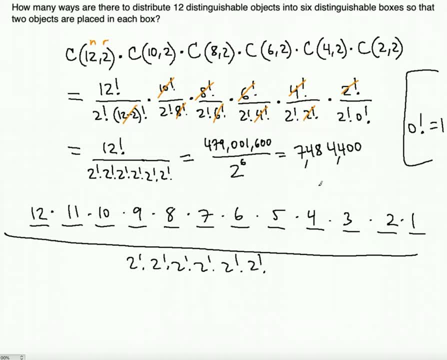 So that's going to be 7,484,400 ways to distribute 12 distinguishable objects into 6 distinguishable boxes, so that 2 objects are placed in each box. So I hope this was fun and helpful. Thanks for watching and I'll see you in the next video.